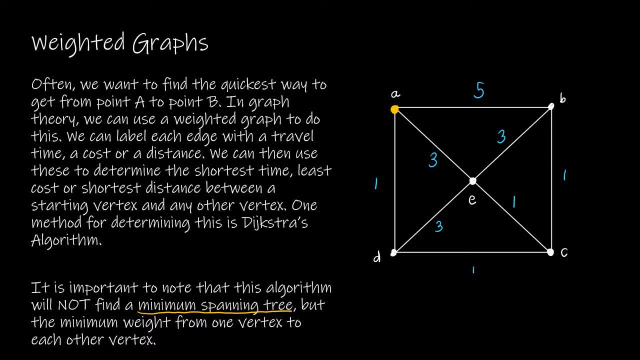 cheapest way in order to visit each other vertex. So it is a little bit different in that this is not a minimum spanning tree. It's not the cheapest way to visit all of the vertices. It's the cheapest way to visit each individual vertex. So I wanted to give you the actual algorithm. 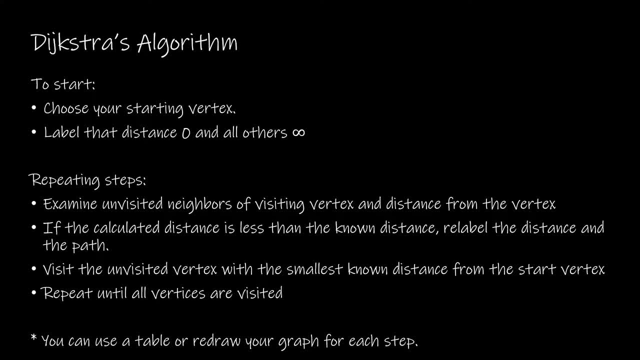 In plain language, just so you understood exactly what it is that we're going to do, And then we're actually going to work through this together. So, to begin, we're going to choose our starting vertex. I've already told you we're going to start with A, So we're going to label that. 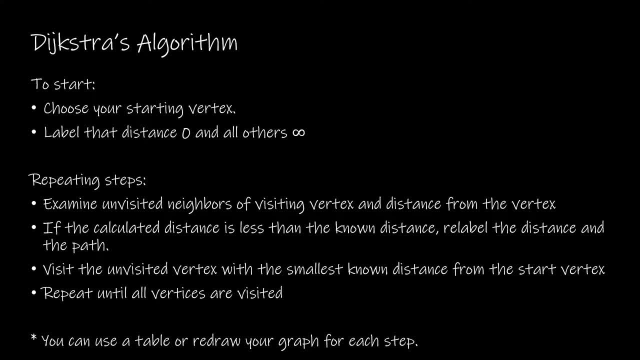 distance zero and all of the other distances we're going to label infinity, because we want it to be a very large number, And eventually we will replace each distance with another distance based on the repeating steps that I've given you. For the repeating steps, we're going to examine any unvisited neighbors from our visiting vertex. 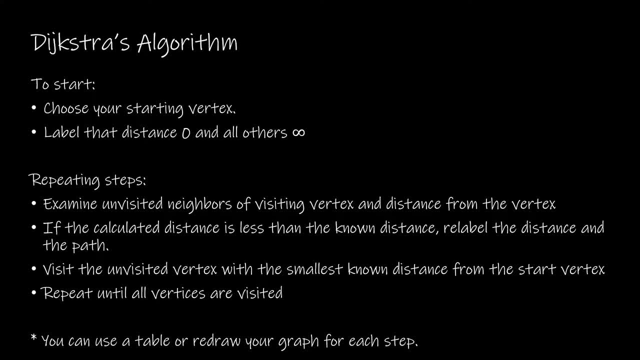 So again, we're going to begin at A, So we're going to look at anything that is connected to A, so any adjacent vertices to A, And we're going to look at the distance from that vertex And if the distance is less than the known distance, so at first it's definitely going to be because our known 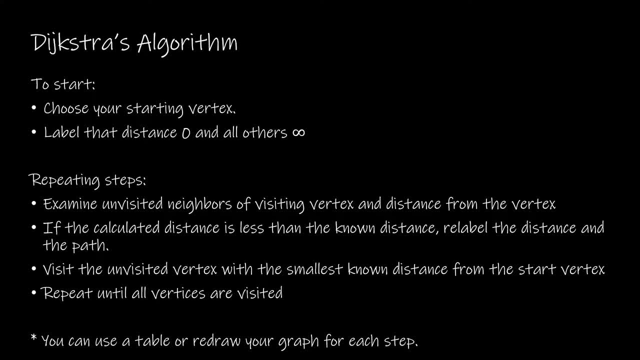 distance is going to be infinity to any other distance, then we're going to relabel the distance itself, And if it's not, we'll leave it as is. And then we're going to visit or choose the unvisited vertex with the smallest known distance from the start vertex, And then we're just going to keep. 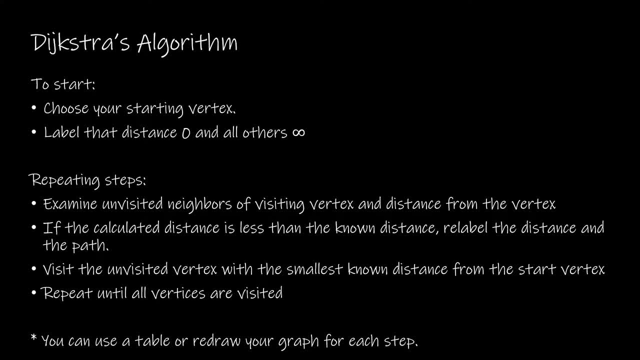 doing that until we have visited every single vertex. Now, different textbooks, different videos you may find on YouTube- have you perform this algorithm in different ways? So it's still the same algorithm, but it might be that you use a table, or it might be that you use a table or it. 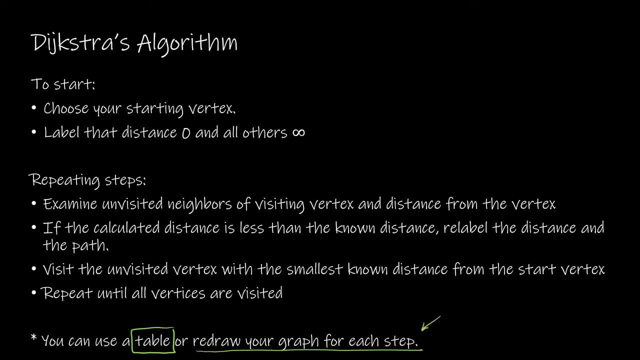 might be that you redraw your graph for each step, So in your textbook it takes you through how to do the redrawing for each step. I'm going to do sort of an abridged version of that, because I'm too lazy to redraw my graph each time, And I'm also going to show you how to use a table, because 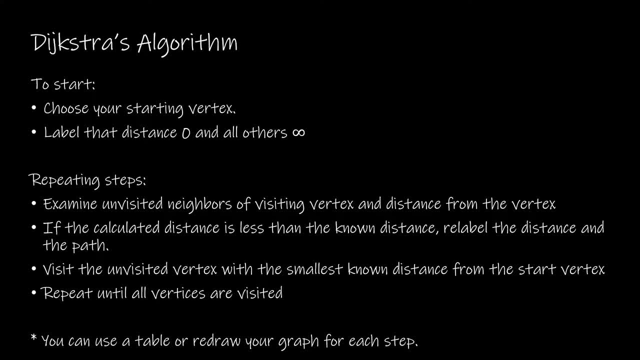 In plain language, just so you understood exactly what it is that we're going to do, And then we're actually going to work through this together. So, to begin, we're going to choose our starting vertex. I've already told you we're going to start with A, So we're going to label that. 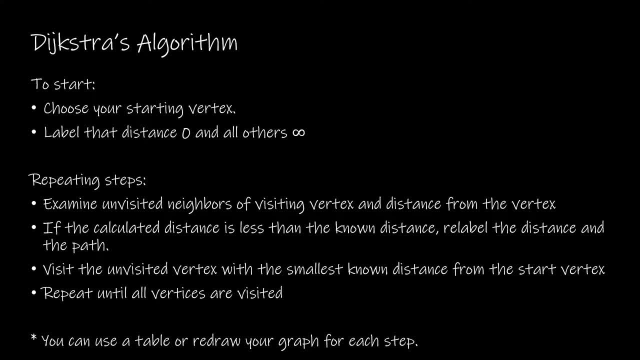 distance zero and all of the other distances we're going to label infinity, because we want it to be a very large number, And eventually we will replace each distance with another distance based on the repeating steps that I've given you. For the repeating steps, we're going to examine any unvisited neighbors from our visiting vertex. 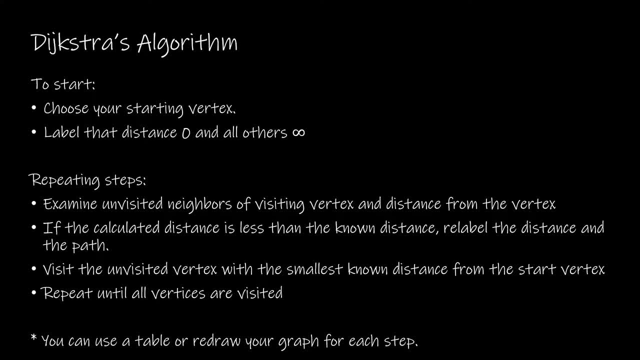 So again, we're going to begin at A, So we're going to look at anything that is connected to A, so any adjacent vertices to A, And we're going to look at the distance from that vertex And if the distance is less than the known distance, so at first it's definitely going to be because our known 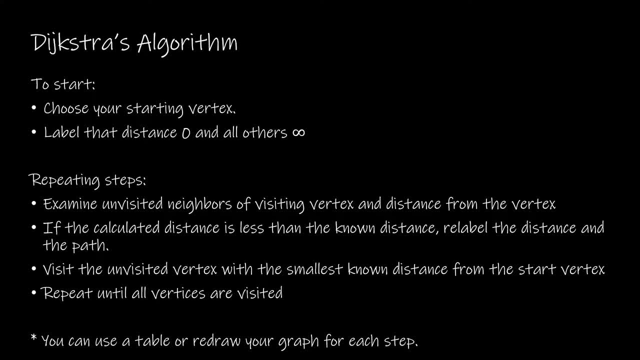 distance is going to be infinity to any other distance, then we're going to relabel the distance itself, And if it's not, we'll leave it as is. And then we're going to visit or choose the unvisited vertex with the smallest known distance from the start vertex, And then we're just going to keep. 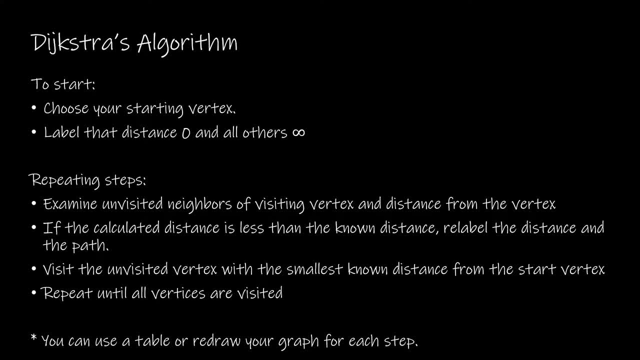 doing that until we have visited every single vertex. Now, different textbooks, different videos you may find on YouTube- have you perform this algorithm in different ways? So it's still the same algorithm, but it might be that you use a table, or it might be that you use a table or it. 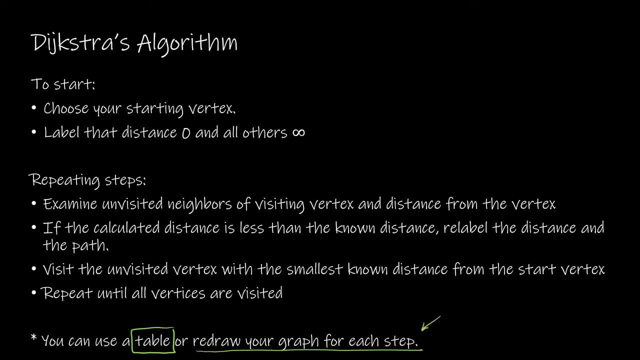 might be that you redraw your graph for each step, So in your textbook it takes you through how to do the redrawing for each step. I'm going to do sort of an abridged version of that, because I'm too lazy to redraw my graph each time, And I'm also going to show you how to use a table, because 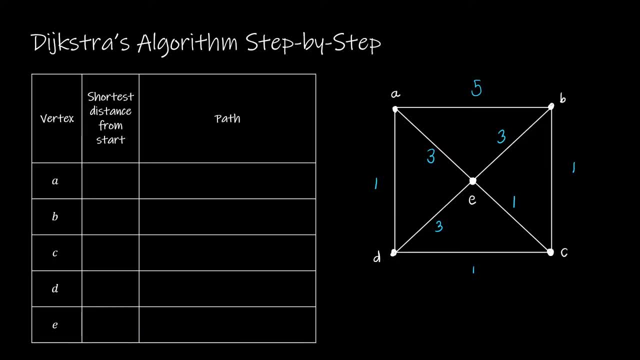 I feel it's probably the easiest way to do it. We're going to do this example step by step And, as we are working through this, I'm going to show you both how I would like you, as my student, to show work on a table or show work on the graph. Now, if you are watching, 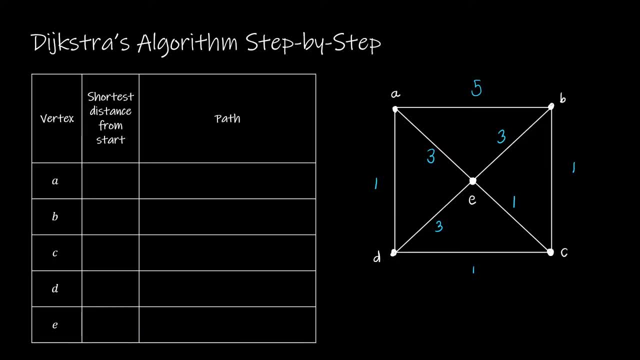 I feel it's probably the easiest way to do it. We're going to do this example step by step And, as we are working through this, I'm going to show you both how I would like you, as my student, to show work on a table or show work on the graph. Now, if you are watching, 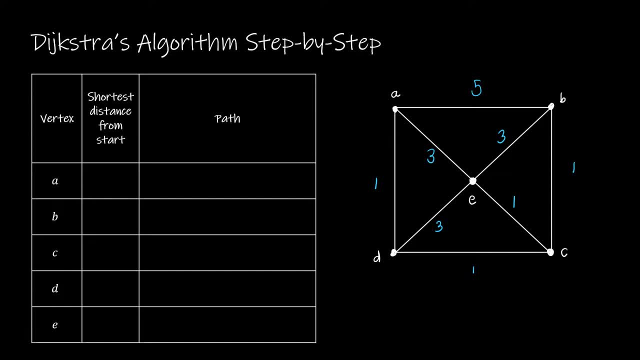 this video on YouTube and I'm not your instructor. I would make sure that you reach out to your instructor to see how he or she would like you to show your work For my students. I do want to see the process involved, So I don't just want to see the final outcome, but I want to see the steps. 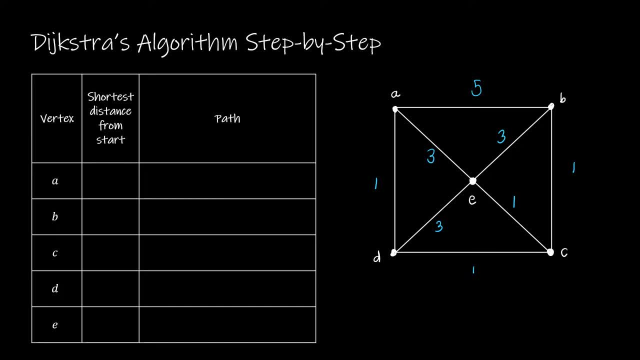 that you took. So that's what I'm going to model here as we go through this example. So, as you can see, I have my weighted graph and we've already determined that I'm going to use the table to show work on the graph and I want to pull that table to show what I did there. So I don't want to see 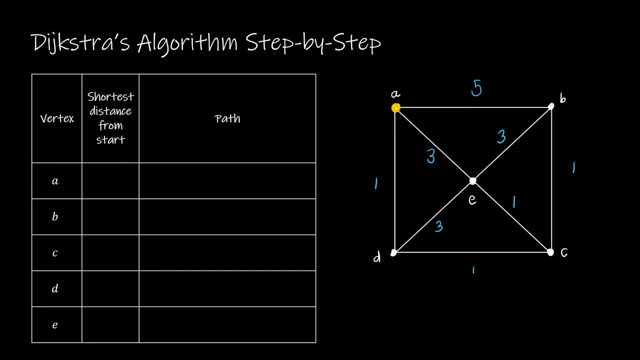 any drawing lines. So before I begin on the table, I want to make sure that I've written down either the first two bars- the first two, unless I didn't want to show it to the distance- and the a after that. You can also pull that down and you can shown that in whatever instance. Again, 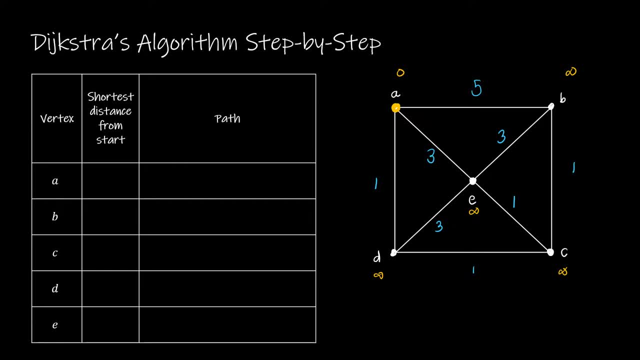 if I take my grade to sqaure or it will not show up on this table. We can talk about A in G, but what I did true so far is I've shown that I'm going to show unscooked appliasa L's typical. 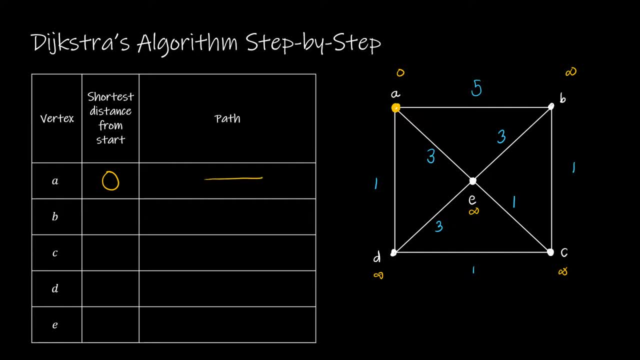 path. So I've shown that I'm going to use my work action method of pulling the table and created a I don't have to worry about, because to get from A to A I didn't go anywhere, But everything else I'm going to use a distance of infinity. 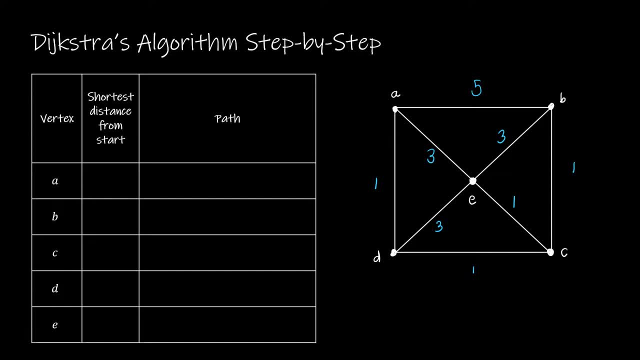 this video on YouTube and I'm not your instructor. I would make sure that you reach out to your instructor to see how he or she would like you to show your work For my students. I do want to see the process involved, So I don't just want to see the final outcome, but I want to see the steps. 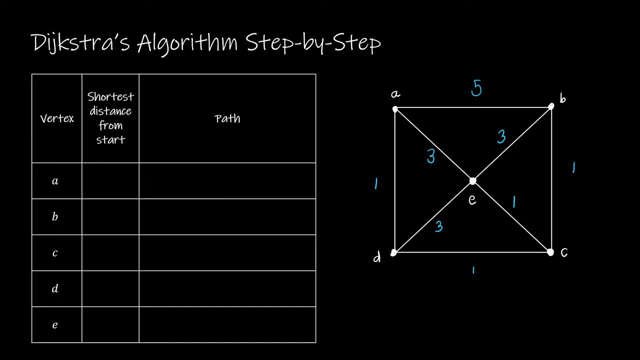 that you took. So that's what I'm going to model here as we go through this example. So, as you can see, I have my weighted graph and we've already determined that I'm going to use the table to show work on the graph using a table. You can see here that I've powered the table up. So here we are. 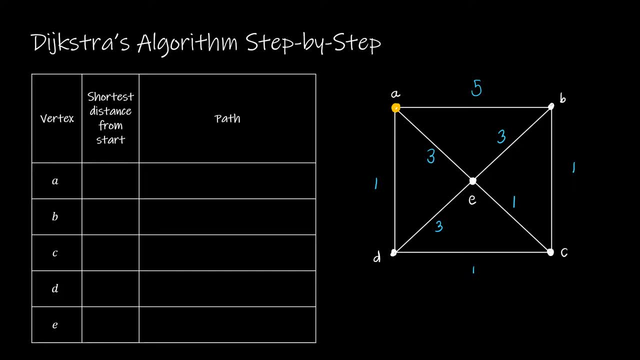 at the end of my seat. right now I'm going to send the table disable and just again start with that oneâu distance at one zone. And what now comes first is that the table set up on top of the of the table. how I can show rate to the graph at one zone. 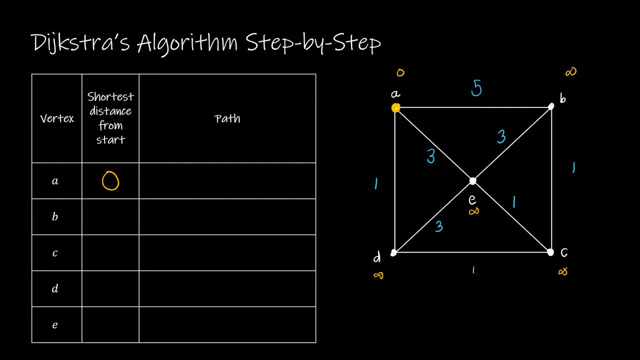 So what we're going to be doing now is that we're going to pass the table off to our students and and the table pops up to us anyway, so that we've taken our table and then superimposed it. So if we are used to using the table names if you'd only want to set up at one zone, for example, no one can do that in an empty table, If you wish. 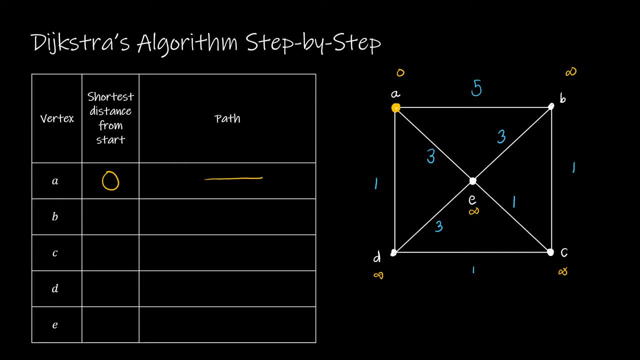 I don't have to worry about, because to get from A to A I didn't go anywhere. But everything else I'm going to use a distance of infinity And if you'll notice, I'm drawing infinity, not super big, because I'm saving room in that table to show the next steps. 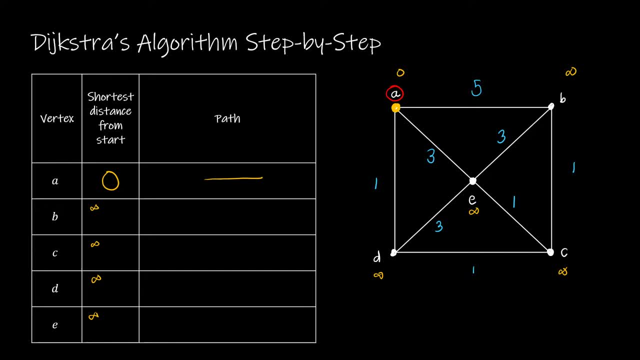 So the next step from A is first to indicate that A has been visited. So I'm just going to circle it to know that it has been visited And then I need to look at any unvisited vertices. So to get from A to B, 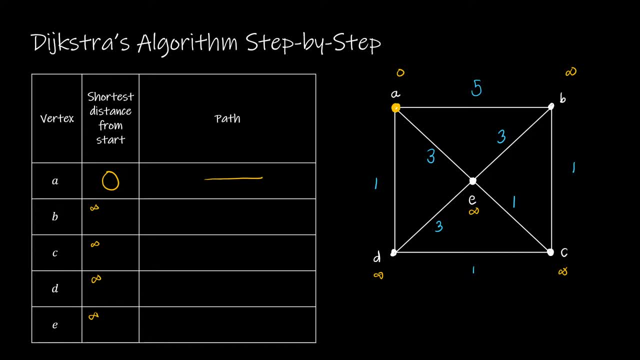 And, if you'll notice, I'm drawing infinity, not super big because I'm saving room in that table to show the next steps. So the next step from A is first to indicate that A has been visited. So I'm just going to circle it to know that it has been visited. 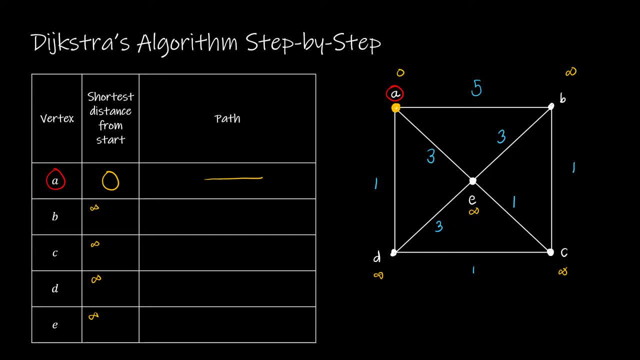 And then I need to look at any unvisited vertices. So to get from A to B, that would take a distance or cost of five. Now, five is kind of a lot, but it is less than infinity. So I'm going to cross off infinity and replace it with a cost of five. 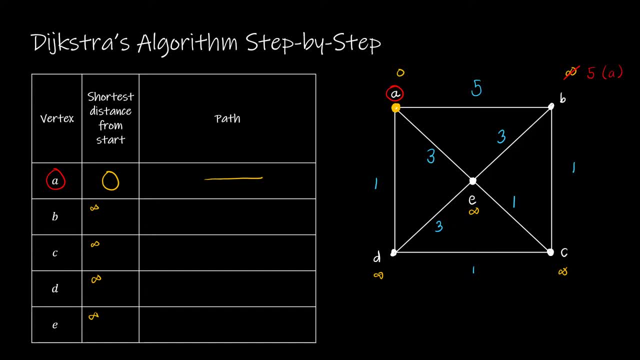 And the path comes from A. And again, I would do the same thing over here. I would replace it with five and a path of A. So, depending on how you're showing work, Then I'm going to look At E. Well, to get to E, I have three coming from A. 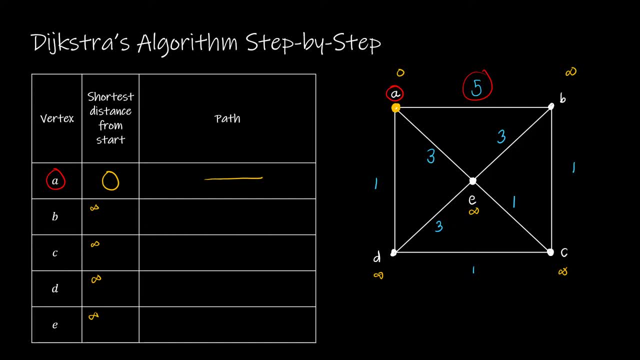 that would take a distance or cost of five. Now, five is kind of a lot, but it is less than infinity. So I'm going to cross off infinity and replace it with a cost of five. And the path comes from A And again. I would do the same thing over here. I would replace it with five. 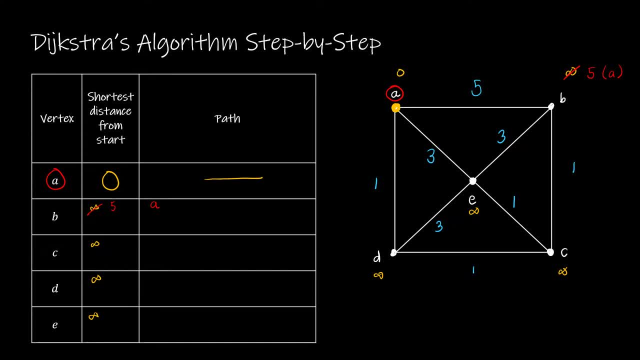 and apply a cost of four And I'm going to cross off infinity and replace it with a cost of five. path of A. So depending on how you're showing work, Then I'm going to look at E. Well, to get. 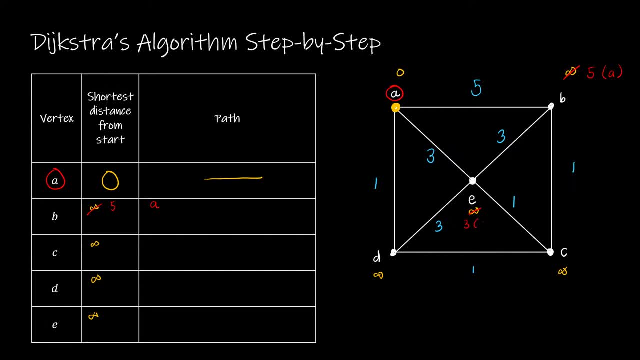 to E. I have three coming from A And again three coming from A, And to get to D is a distance of one coming from A. So D is one and A. The next step is to choose which vertex I would not like. 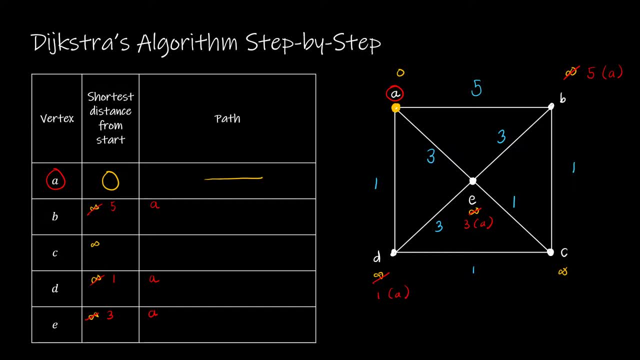 to next visit, And the next visiting vertex should be the cheapest one or the shortest one, whatever the least amount is, So we can tell very easily that that is one for D. So I'm going to visit D And that means that again, the shortest distance is one and that path is A D. 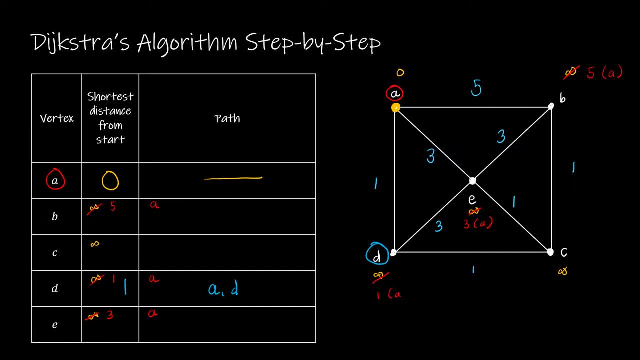 And again, I can either write A, D here. I typically just leave it as A if I'm showing it there Now I have to look at each distance. I shouldn't have used blue. That might get confusing, but we're going to go with it. I have to look from. 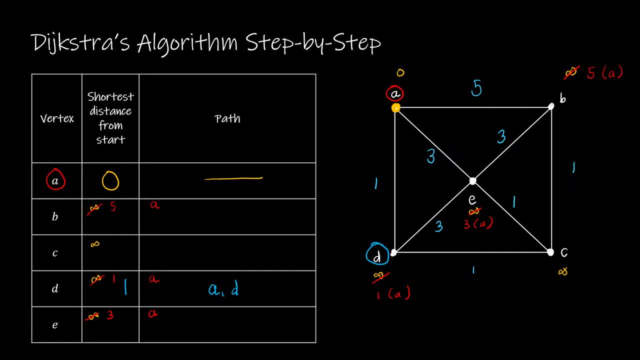 D to each unvisited vertex. So, as you can see, E has already been relabeled as 3A, but it's not a visited vertex. It's still an unvisited vertex because I've only visited A and D so far. Whoops, I should circle D. 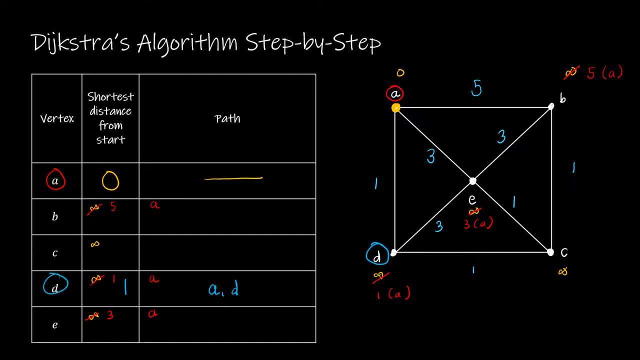 Right here. So now I'm going to look at E And to get to E from D would have a distance of 1 plus 3. So that's a distance of 4.. Now 4 happens to be greater than the 3. that's already. 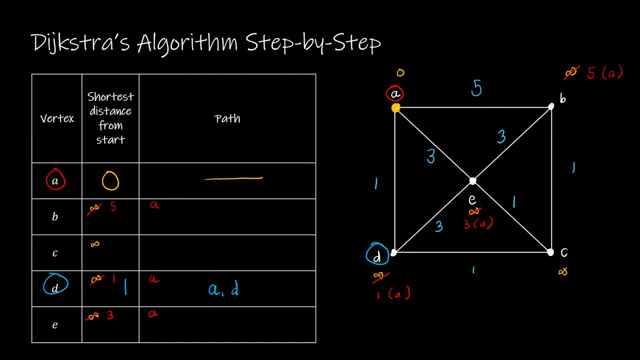 there. So I'm not going to relabel E, because we're only going to relabel if the cost is less. Then the other unvisited vertex is C and that would have a distance of 1 plus 1, or 2.. So I'm going to look at E and to get to E from D would have a distance of 1 plus 3.. So 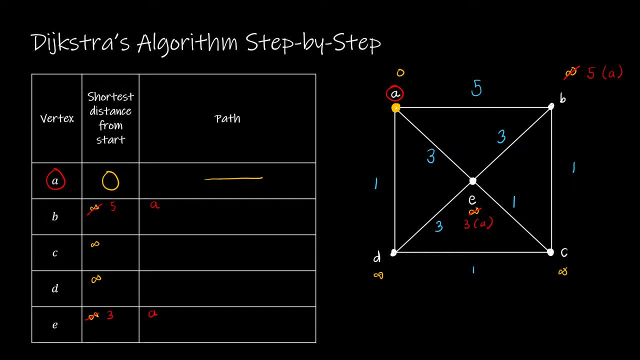 And again three coming from A, And to get to D is a distance of one coming from A, So D is one and A. The next step is to choose which vertex I would not like to next visit, And the next visiting vertex should be the cheapest one or the shortest one. 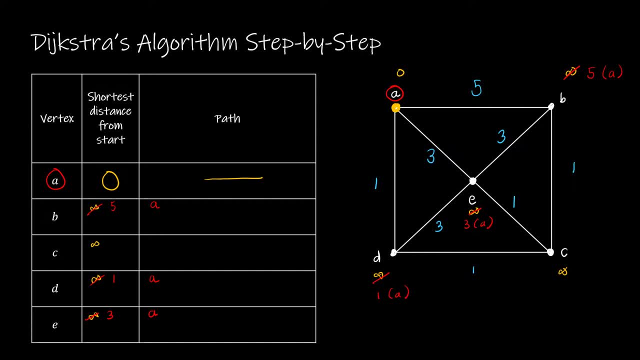 Whatever the Least amount is. So we can tell very easily that that is one for D. So I'm going to visit D And that means that again the shortest distance is one And that path is A D, And again I can either write A D here. 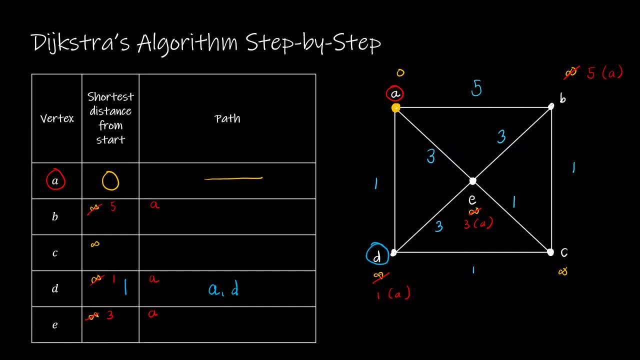 I typically just leave it as A. if I'm showing it there Now, I have to look at each Distance. I shouldn't have used blue, That might get confusing, but we're going to go with it. I have to look from D to each unvisited vertex. 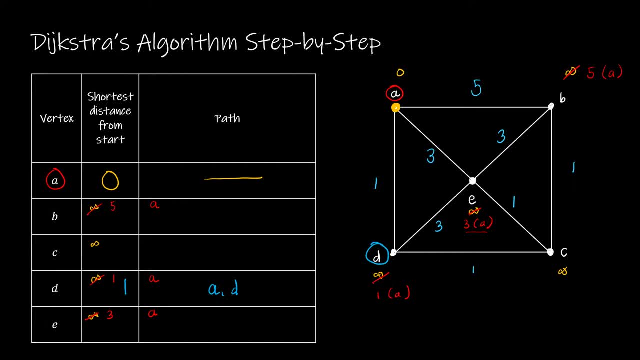 So, as you can see, E has already been relabeled as three A, but it's not a visited vertex. It's still an unvisited vertex because I've only visited A and D so far. Whoops, I should circle D right here. 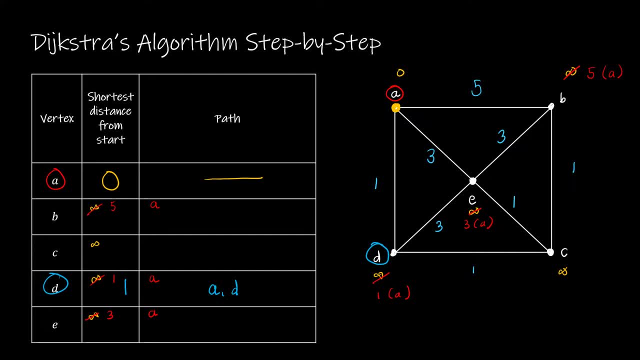 So now I'm going to look at E and to get to E from D. So we have a distance of one plus three, So that's a distance of four. Now four happens to be greater than the three. that's already there. So I'm not going to relabel E, because we're only going to relabel if the cost is less. 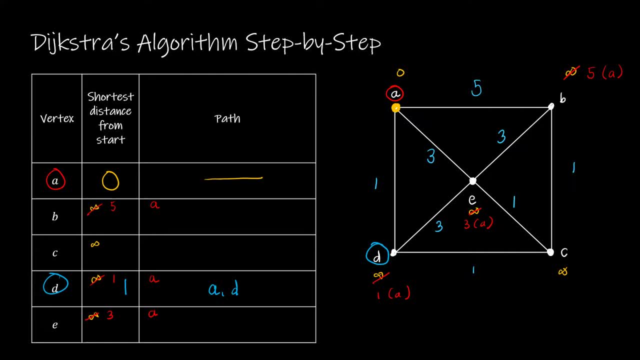 Then the other unvisited vertex is C, and that would have a distance of one plus one or two. So this is two comma A- D. So from here. I'm going to look- I'm sorry I should have replaced it over here as well- to AD From here. 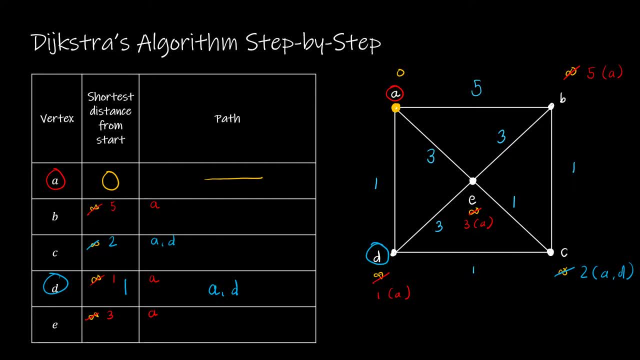 I'm going to look at any of the unvisited vertices and determine which is cheapest to get to, And that answer is C. To get to C, I'm going to take A to D. So now my cost is 2 and my path is AD. 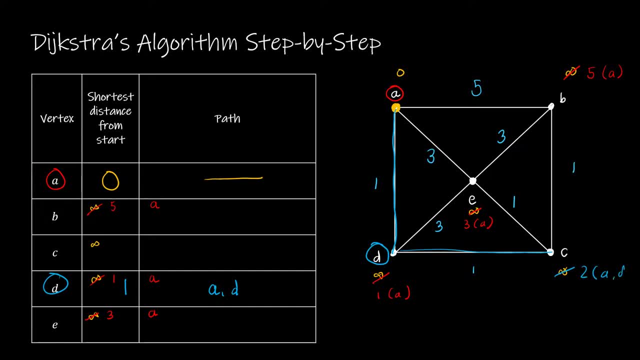 this is 2, A D, So from here I'm going to look. I'm sorry, I should have replaced it over here as well. 2, A D. From here I'm going to look at any of the unvisited vertices. 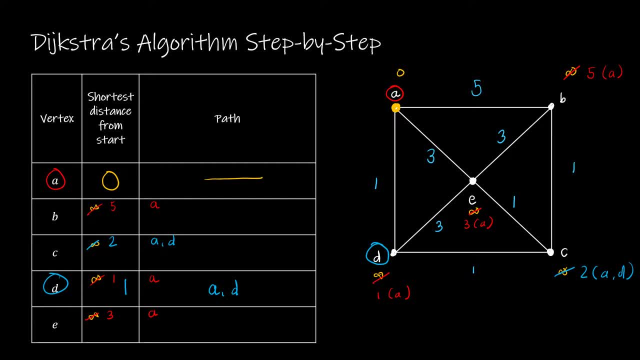 and determine which is cheapest to get to, And that answer is C. To get to C, I'm going to take A to D, So now my cost is 2.. So I'm going to look at any of the unvisited vertices and determine. 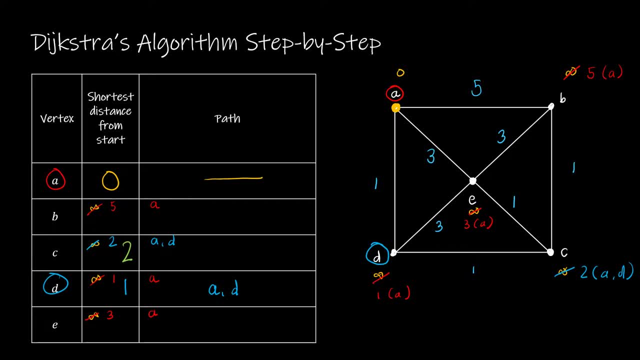 which is cheapest to get to? And that answer is 2.. So now my cost is 2.. So now my cost is 2.. And my path is A, D, and I'm just going to write A D, C, A D C. Now, whether or not you include the C, 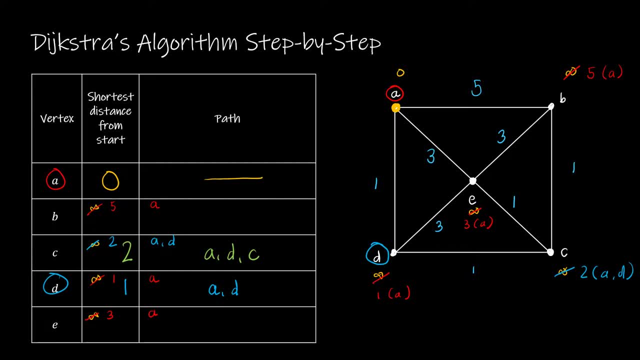 is sort of up to you. I find it easier to include the C, But again, as you can see over here, I only have A, D, So now I have visited C and I only have two more unvisited vertices of B and E. 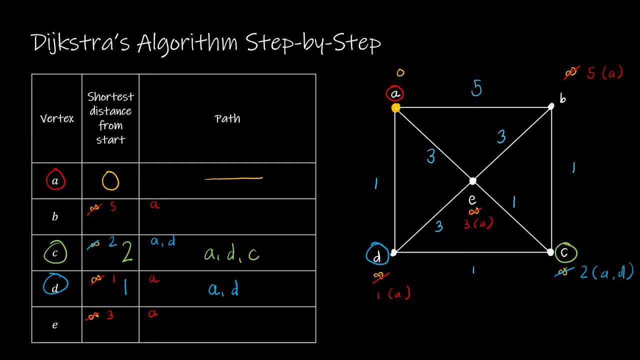 Coming from C. I now have to look at those two unvisited vertices and see if I can change any of the values. So to get to E from C, I would have a distance of 2 plus 1, which is 3.. Now 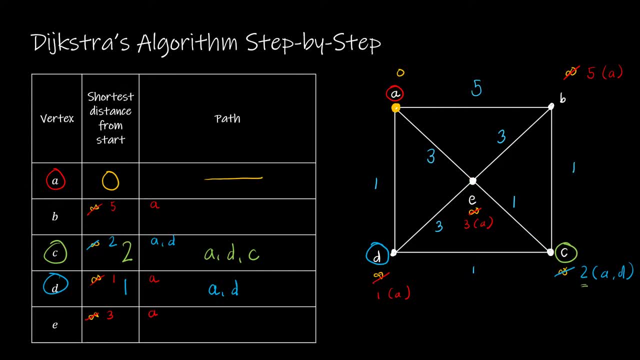 3 is the same as 3.. So I'm just going to leave it as is. To get from C to B would have a distance of 3.. So I'm just going to leave it as is. To get from C to B would have a distance of 3.. So 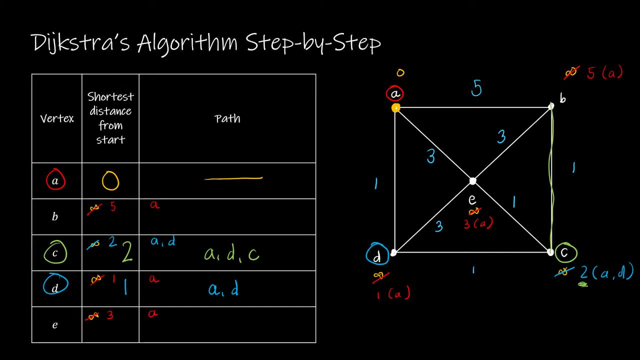 to get from C to B would have a distance of 2 plus 1, which is 3.. Well, 3 is less than 5.. So I'm going to replace 5 with 3.. And instead of going straight from A, we went from A to D to C. 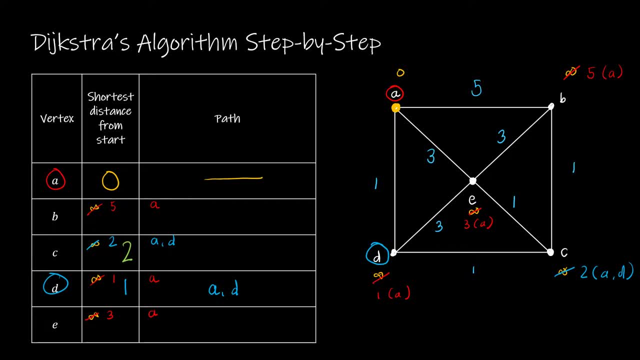 and I'm just going to write ADC, ADC. Now, whether or not you include the C is sort of up to you. I find it easier to include the C, But again, as you can see over here, I only have AD. 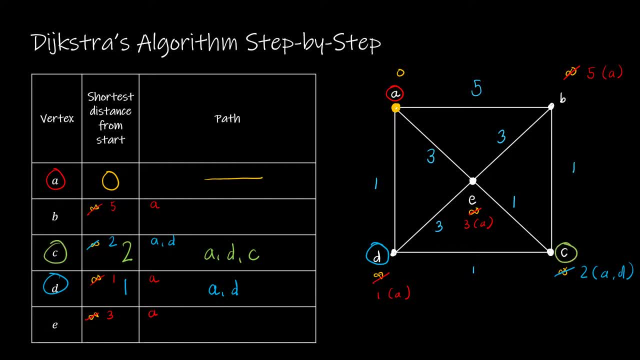 So now I have visited C and I only have two more unvisited vertices of B and E Coming from C. I now have to look at those two unvisited vertices and see if I can change any of the values. So to get to E from C I would have a distance of 2. 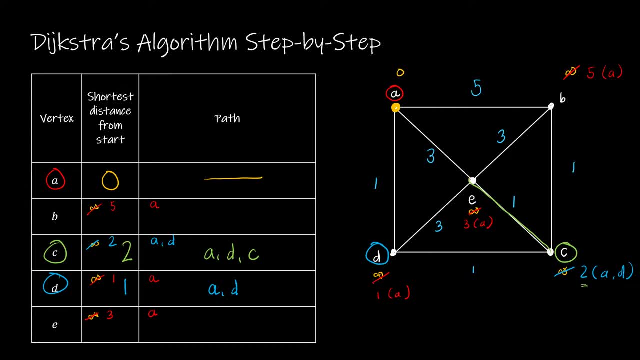 plus 1, which is 3.. Now, 3 is the same as 3, so I'm just going to leave it as is. To get from C to B would have a distance of 2 plus 1, which is 3.. Well, 3 is the same as 3,. 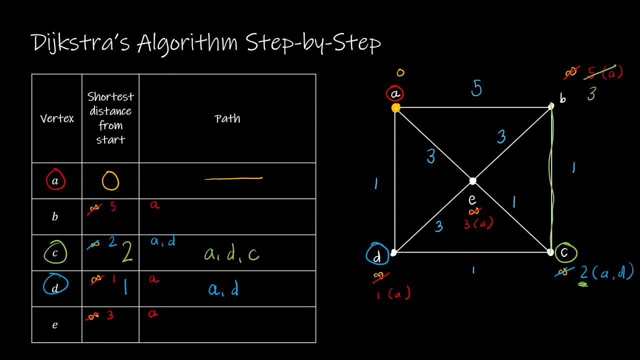 less than 5.. So I'm going to replace 5 with 3.. And instead of going straight from A, we went from A to D to C. So now B is replaced with 3, and A is replaced with ADC. So now what? Well, now I have to choose a vertex to visit. Now you can see both B and E. 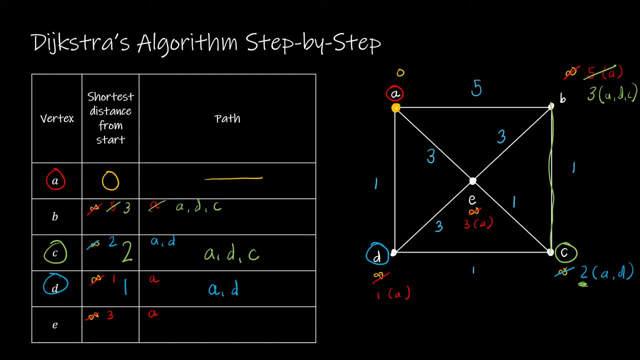 have a cost of 3, or distance of 3.. And so it really doesn't matter which one I choose, because it's going to be the same. So I'm going to go ahead and choose B to visit. So B has been visited. The cost is 3.. The path is ADCB, Or you can leave it just as is up here. 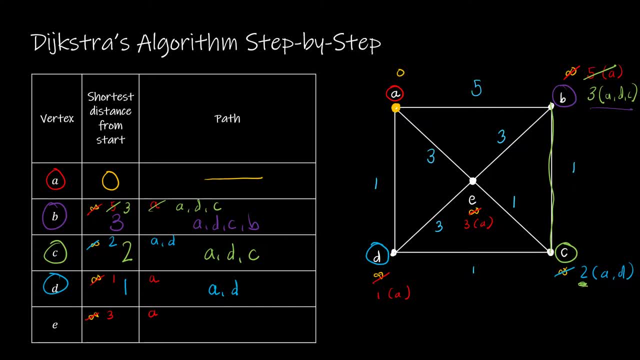 3 ADC, And then, of course, the last one is E. So we're going to visit E and that has a cost of 3. And then that's AE or just 3A. So, as you can see, it's kind of the same process. 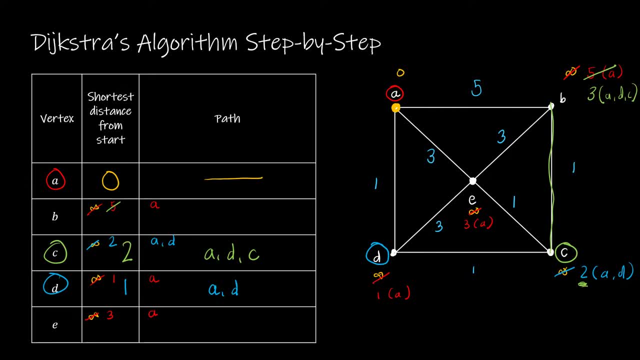 So now B is replaced with 3, and A is replaced with A, D, C. So now what? Well, now I have to choose a vertex to the right of the vertex. So now I have to choose a vertex to the left of the vertex. So, 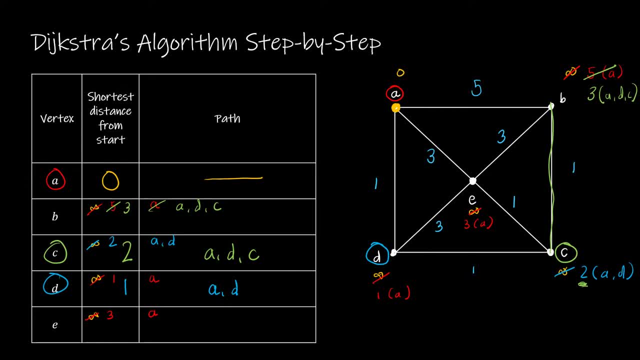 I'm going to go ahead and choose B to visit. Now you can see both B and E have a cost of 3, or distance of 3.. And so it really doesn't matter which one I choose, because it's going to be the. 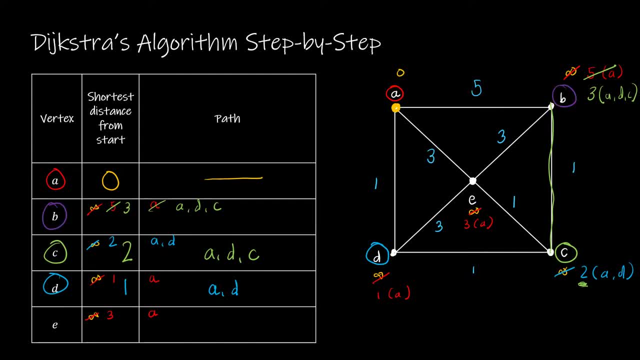 same, So I'm going to go ahead and choose B to visit. So B has been visited. The cost is 3.. The path is A D, C, B Or you can leave it just as is up here. 3, A D, C. 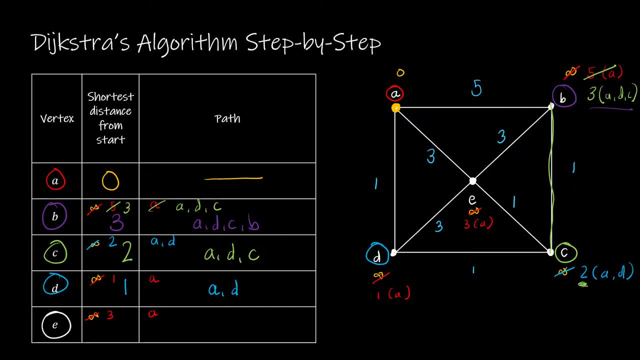 And then, of course, the last one is E. So we're going to visit E and that has a cost of 3.. And then that's A E or just 3, A. So, as you can see, it's kind of the same process. 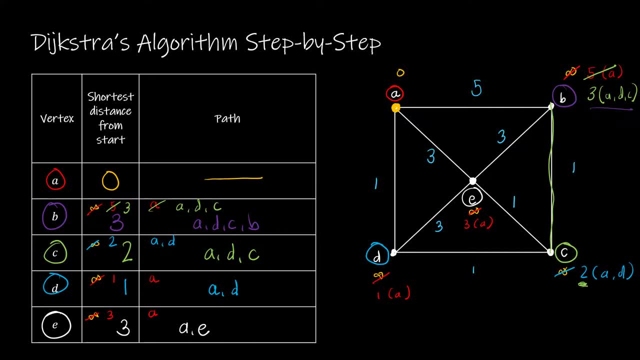 whether I'm using a table or a graph, And this tells me: from A, the shortest path to B is a distance of 3, and we go from A to D to C, to B. To get to C, the shortest path is 2, or distance is 2, and the path is A, D, C. 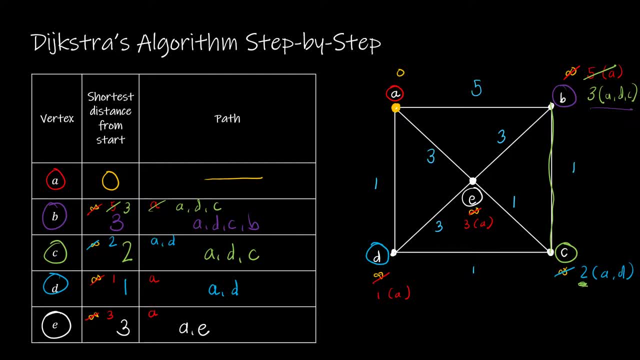 To get to D, the shortest path is 1, and that's just straight from A to D. And to get to E, the shortest path is 3, and that's from A to E. Here's a question for you to practice on your own, So try this question When you're ready. 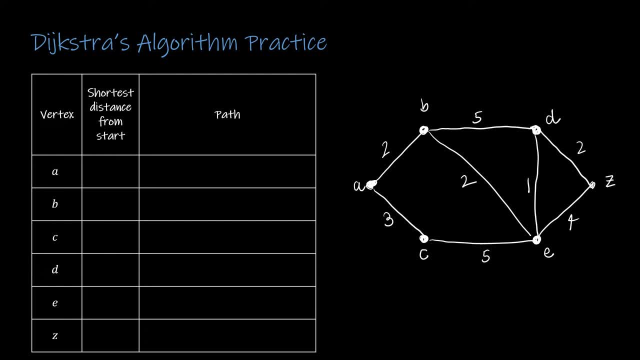 press play to see how you did. Again, we're going to begin at A. I should have made that clear from the beginning. but the distance to get to A is 0, and all of the other distances are infinity. So so far, so good. Now I'm going to choose A. I'm going to say, okay, I did choose A, I'm going. 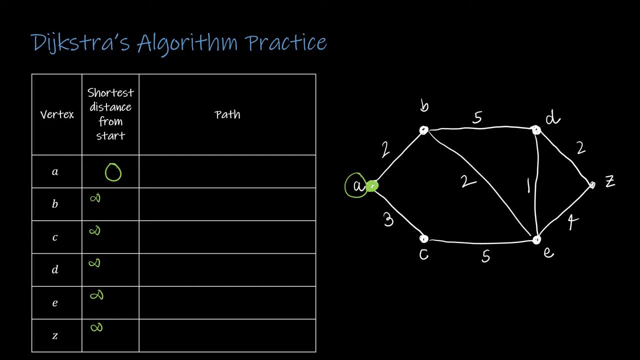 to start there. I have visited A. Where can I get to from that visited vertex? So the visited vertex is A and I can get to either B, which is a distance of 2.. So I'm going to replace infinity. 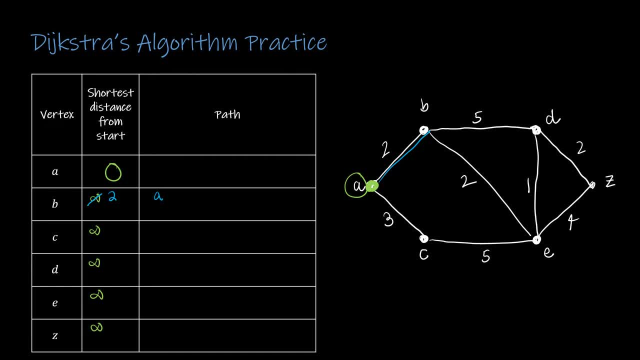 with 2.. So this is coming from A And if you want, you can write AB. You might also see videos out there that just have you write the previous vertex, which is a little bit cleaner, but you have to do a little bit more work to find the path. So if I just, I'll just put these over here. 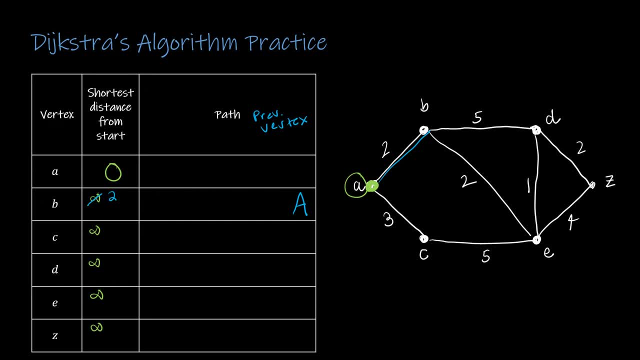 just so you can see one more way in which you can show this work. But B has a weight of 2, coming from A and C is a distance of 2.. So if I just put A and B together I can get to A. 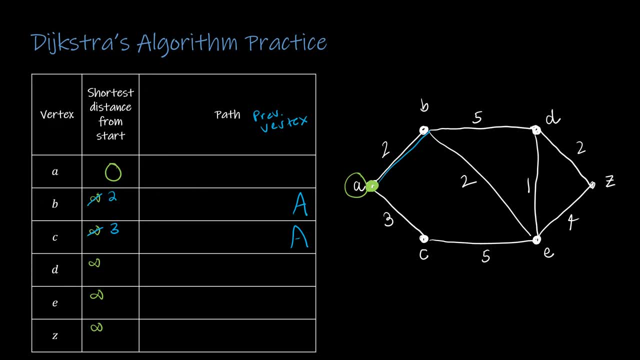 So if I just put A and B together I can get to. A and B is a distance of 2.. So if I just put A and B together, has a weight of three coming from a or again, the path would be a- c or the path would be a- b. 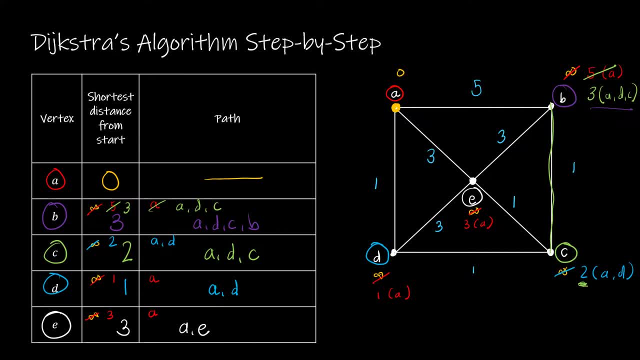 whether I'm using a table or a graph, And this tells me: from A, the shortest path to B is a distance of 3.. And we go from A to D to C, to B. To get to C, the shortest path is 2,. 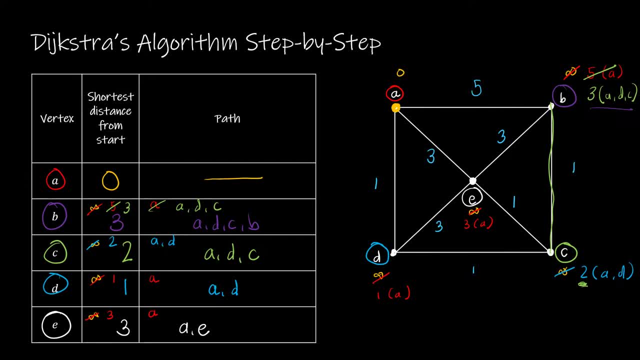 or distance is 2.. And the path is 3.. And then we go from A to D to C to B, And we go from A to D to C to B To get to D, the shortest path is 1, and that's just straight from A to D. And to get to E, 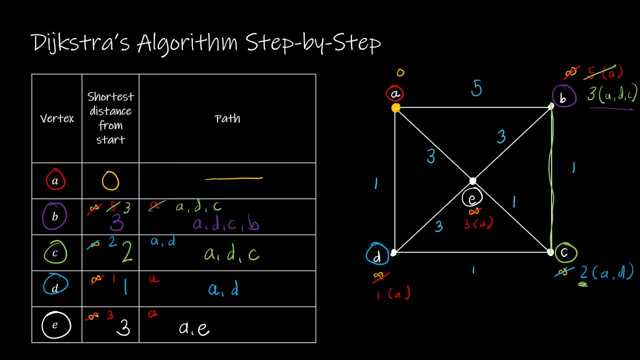 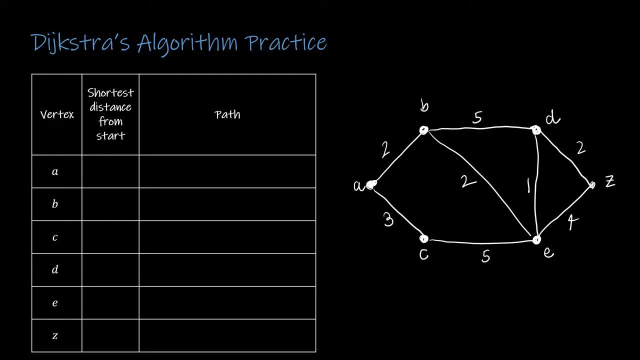 the shortest path is 3, and that's from A to E. Here's a question for you to practice on your own, So try this question When you're ready. press play to see how you did. Again, we're going to begin at A. I should have made that clear from the beginning. 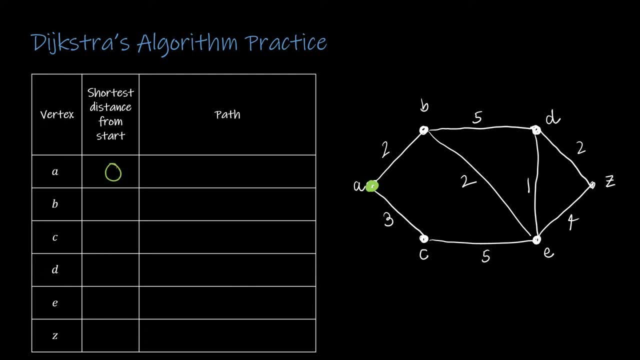 but the distance to get to A is 0. And all of the other distances are infinity. So so far, so good. Now I'm going to choose A and say, okay, I did choose A. I'm going to start there. I have visited A. Where can I get to from that visited vertex? So the visited 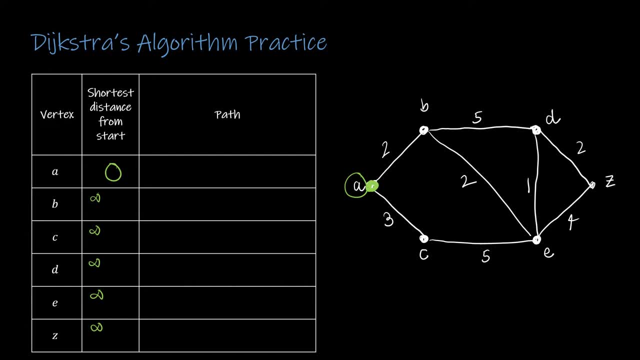 vertex is A and I can get to either B, which is a distance of 2.. So I'm going to replace infinity with 2, coming from A, And if you want, you can write AB. You might also see videos out there that just have you write the previous vertex. 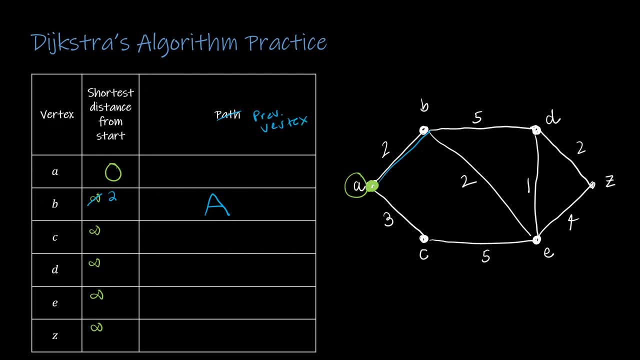 which is a little bit cleaner, but you have to do a little bit more work to find the path. So if I just, I'll just put these over here, just so you can see one more way in which you can show this work. But B has a weight of 2, coming from A, and C has a weight of 3, coming from A. 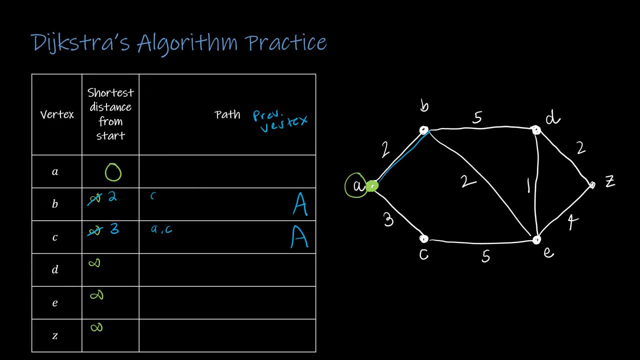 Or again, the path would be AC or the path would be AB. Now, from here, what am I going to do? I'm going to find the cheapest path. So the fastest or cheapest way is to get to B, because 2 is less. 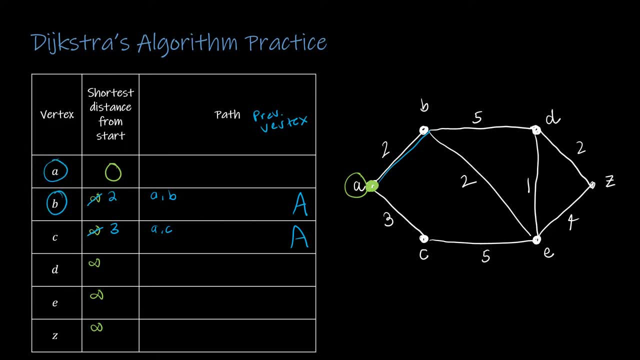 than 3.. So I'm going to choose B. I should have circled that A already, So I visited A. I'm now visiting B, And again B has a distance of 2, and a path of AB or a previous vertex of A. 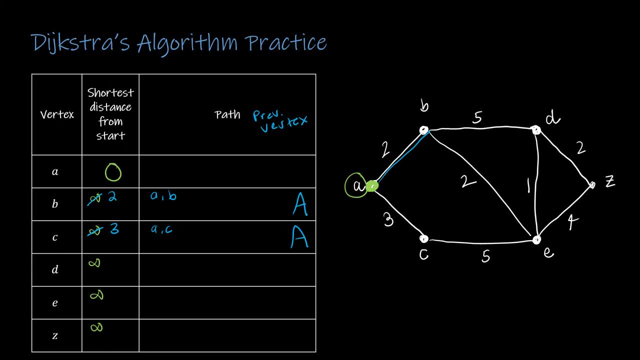 now, from here, what am i going to do? i'm going to find the cheapest path. so this fastest or cheapest way is to get to b, because 2 is less than 3, so i'm going to choose b. i should have circled that a already, so i visited a. i'm now visiting b, and again b has a distance of two. 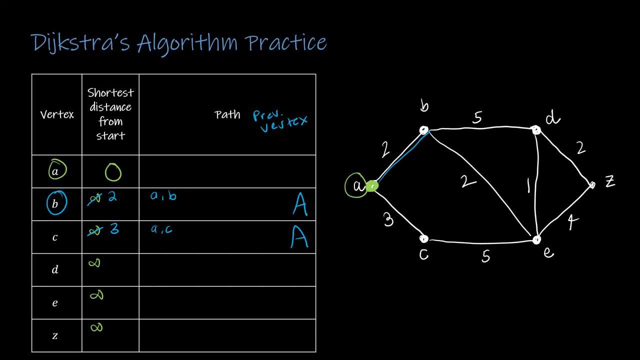 and a path of a, b or a previous vertex of a. so from b i'm now going to look at any adjacent vertices. so from b i can get to d, which would be 2 plus 5 or 7. so d is going to be replaced with 7. 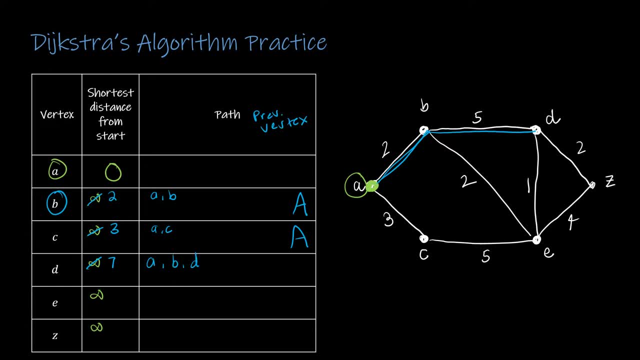 and that path is a, b, d or a previous vertex of b, depending on how you'd like to show your work. i could also get to e. e would be a path of 2 plus 2, which is 4.. and that path would be a to b to e or a previous vertex of b. 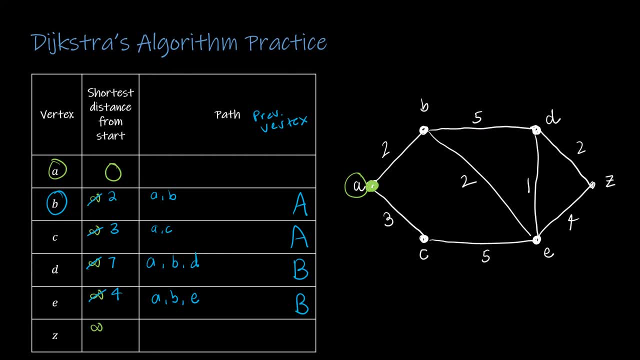 i can't get anywhere out, so z is still not attainable from where i'm standing. so i can't get anywhere out, so z is still not attainable from where i'm standing. so now i'm going to choose what is the cheapest vertex next, so that in this case is c because 3. 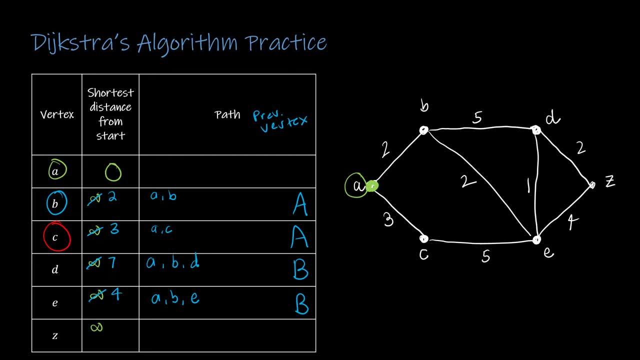 is the lowest number, so i keep forgetting this circle thing. so i'm going to choose c, and c is going to be the next vertex that i visit. so we now have 3 and then ac locked in, and now i'm going to look at any vertices adjacent to c. so c 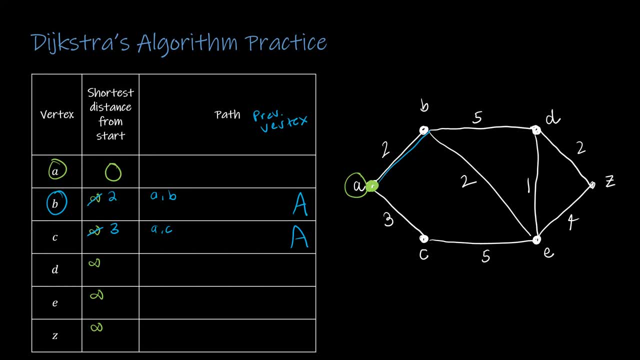 So from B- I'm now going to look at any adjacent vertices- So from B I can get to D, which would be 2 plus 5, or 7.. So D is going to be replaced with 7,, and that path is ABD. 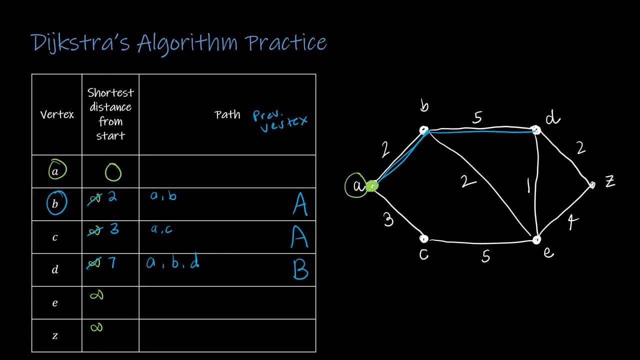 or a previous vertex of B, depending on how you'd like to show your work. I could also get to E. E would be a previous vertex of B, or a previous vertex of B, or a path of 2 plus 2, which is 4.. And that path would be A to B, to E or a previous vertex of B. 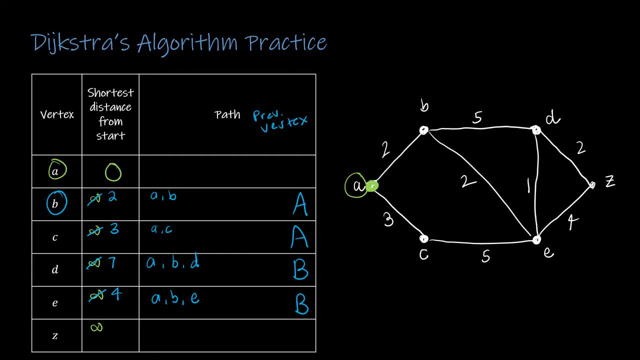 I can't get anywhere out, so Z is still not attainable from where I'm standing. So now I'm going to choose what is the cheapest vertex next. So that in this case is C, because 3 is the lowest number. 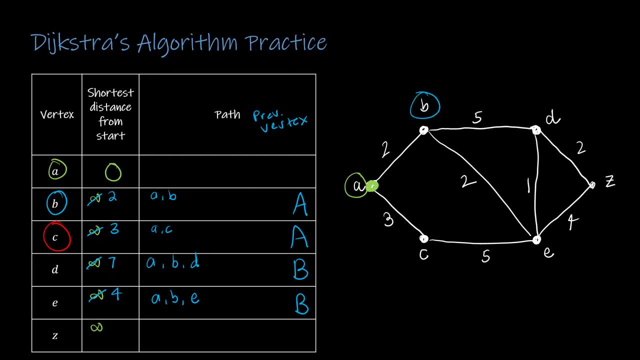 So I keep forgetting this circle thing. So I'm going to choose C, And C is going to be the next vertex that I visit. So we now have 3 and then AC locked in, And now I'm going to look at any vertices adjacent to C, So C can get to E Now that 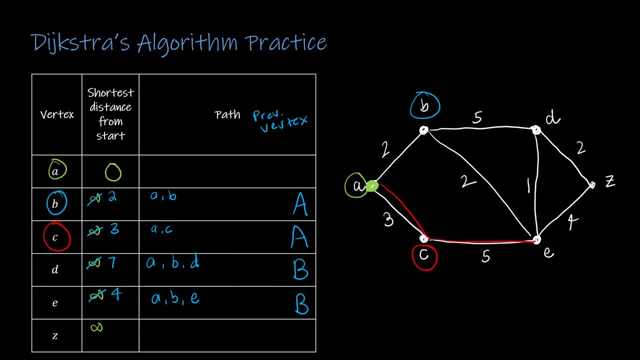 path would be 3 plus 5, which is 8. And currently E has a path or a weight of 4.. So I'm not going to relabel E because it would just be more expensive or more time or more distance. 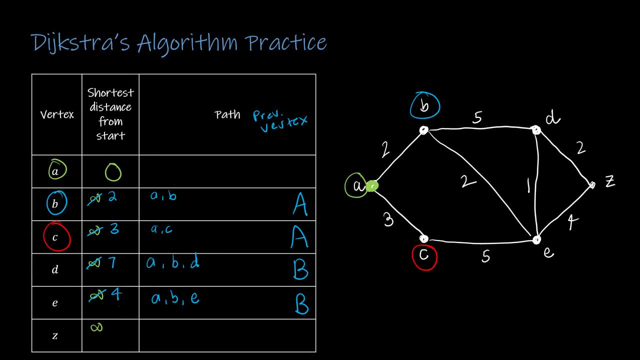 So now I'm just looking at 4 and 7 and saying which one's smaller, 4 or 7? So obviously 4 is smaller, So I'm going to choose E. So E has now been visited with a distance of 4 and a path of ABE, And I'm going to relabel any vertices that I can't. 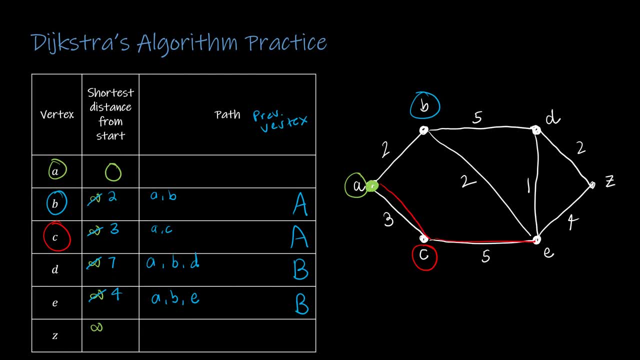 can get to e. now that path would be 3 plus 5, which is 8, and currently e has a path or a weight of 4.. so i'm not going to re-label e because it would just be more expensive or more time or more distance. so now i'm just looking at 4 and 7. 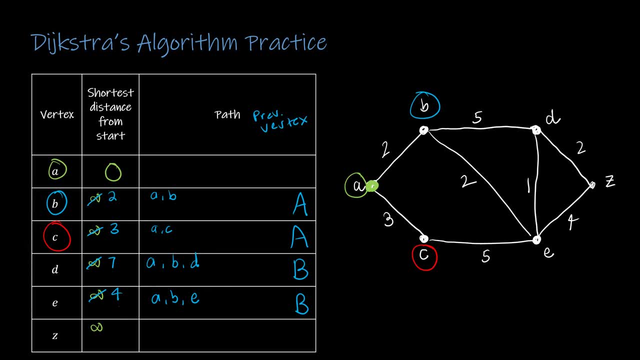 and saying which one's smaller, four or seven. so obviously four is smaller, so i'm going to choose e. so e has now been visited with a distance of 4 and a path of a, b, e and i'm going to re-label any vertices that i can. so to get to d, i would have the four that it takes to get to e, plus one. 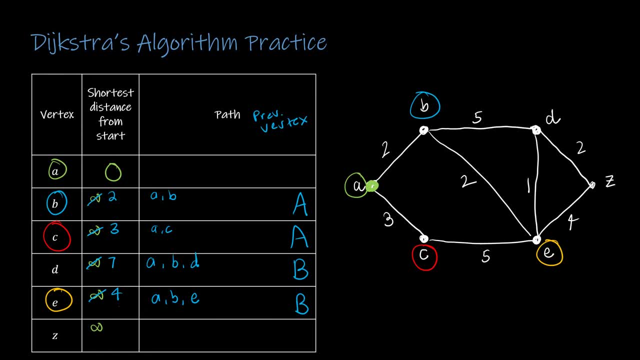 So, to get to D, I'm going to choose E And I'm going to choose E. So I'm going to choose E And I'm going to choose E. I would have the 4 that it takes to get to E, plus one more which is a distance of 5 total. 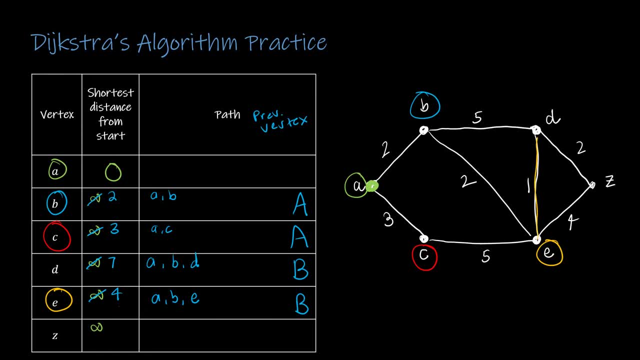 more, which is a distance of five total. currently the distance is seven, so five is better than seven. so i'm re-labeling d with five and that new path is a, b, e, d and that's where the new path is d, or the new previous vertex is that it's coming from e. 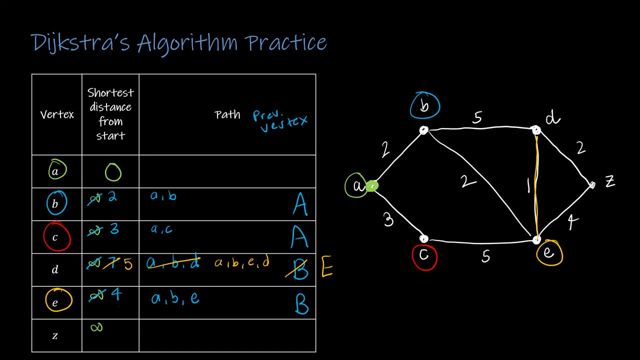 now i'm looking oh. and then i have to look at z and say, can i re-label z? well, yes, i can. so from to get to e was four plus it's four more to get to z. so now z is getting replaced with four plus four or eight and that is a b e z. 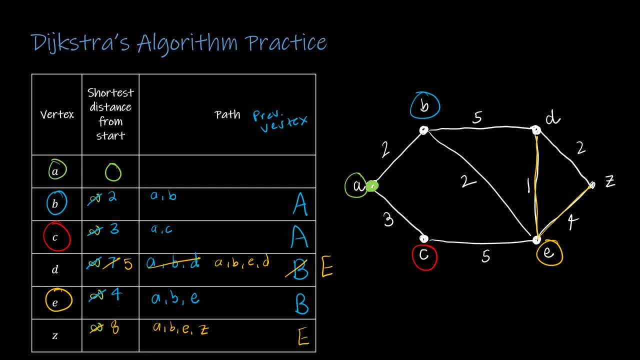 or previous vertex of e. now i'm going to look at the five and the eight and choose the smallest of five and eight, which is, of course, five. i'm trying to find a color we haven't used and i'm striking out: oh, purple. so i'm going to choose five. so now i'm choosing d to visit. d has a weight of. 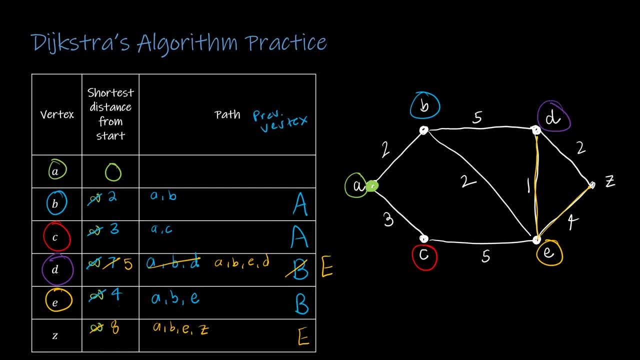 five. the path was a, b, e, d or a previous vertex of e, and the only thing i have left to do is either choose z to be eight or see if i can get to z faster going through d. so to get to d was a weight of five and to get from d to z is two. so five plus two is seven, and seven is better than eight. 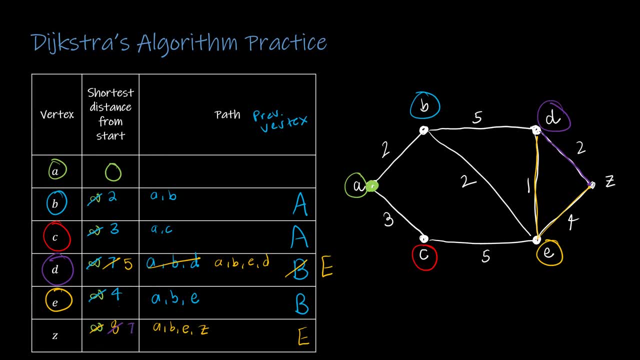 so i'm going to replace eight with seven, and this path now becomes- because i'm coming from d, a, b, e, d, z, or a previous vertex of d. so now i've done it, i've found the cheapest path, and of course then i would choose z. so 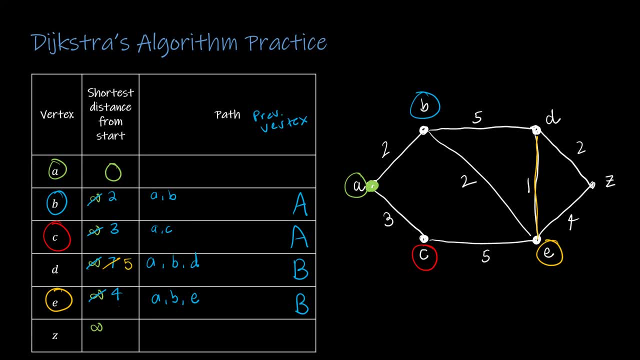 Currently the distance is 7, so 5 is better than 7.. So I'm relabeling D with 5, and that new path is A, B, E, D, or the new previous vertex is that it's coming from E. 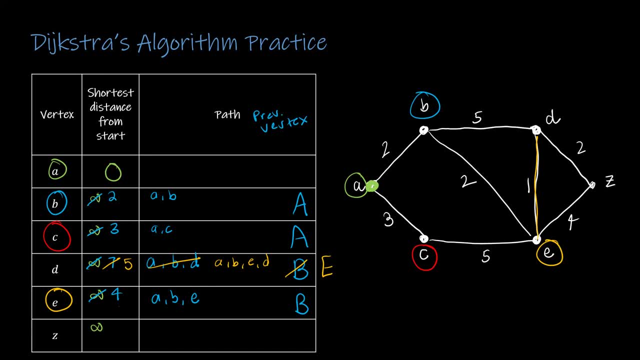 Now I'm looking oh, and then I have to look at Z and say, can I relabel Z? Well, yes, I can. So to get to E was 4, plus it's 4 more to get to Z. 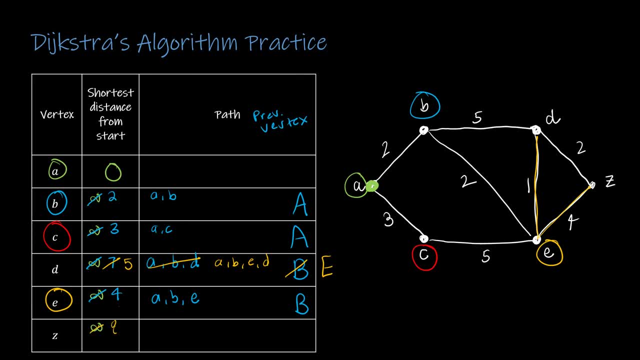 So now Z is getting replaced with 4 plus 4, or 8,, and that is A, B E, Z, or previous vertex of E. Now I'm going to look at the 5 and the 8. And choose the smallest of 5 and 8,, which is, of course, 5.. 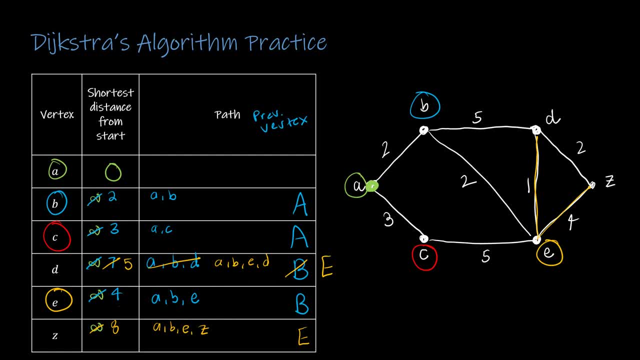 I'm trying to find a color we haven't used and I'm striking out: Oh, purple. So I'm going to choose 5.. So now I'm choosing D to visit. D has a weight of 5.. The path was A, B, E, D or previous vertex of E. 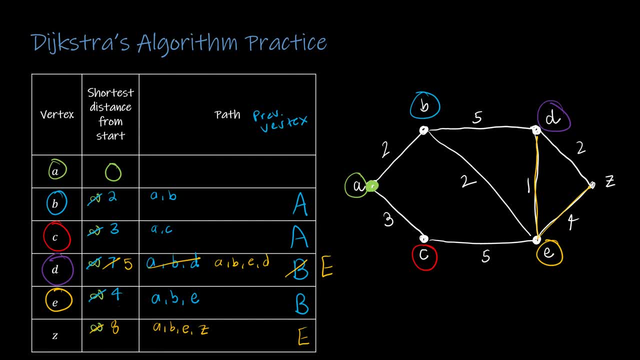 And the only thing I have left to do is either choose Z to be 8, or see if I can get to Z faster going through D. So to get to D was a weight of 5. And to get from D to Z is 2.. 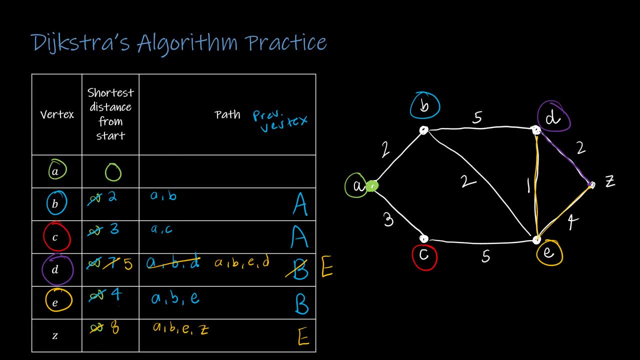 So 5 plus 2 is 7. And 7 is better than 8.. So I'm going to replace 8 with 7.. And this path now becomes- because I'm coming from D, A, B, E, D, Z, or a previous vertex of D- 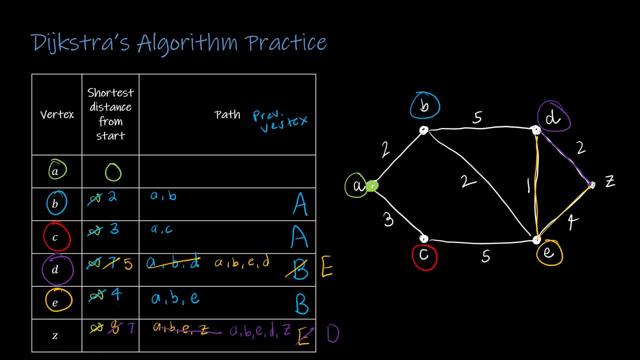 So now I've done it, I've found the cheapest path, And of course, then I would choose Z, So I found the cheapest path to each of these vertices. So if I needed to get from A to D, the cheapest is 5, with A, B, E, D as the path. 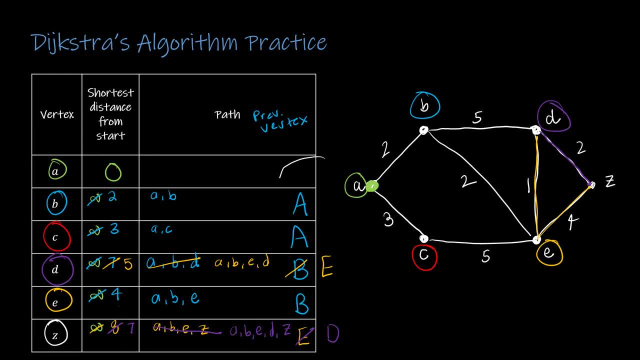 Or again, if you're just looking at the previous vertex. so if you're just showing this, you can find the path. You would just have to do some backtracking. So let's say I was focused on Z. Z says: okay, you had to get to D. 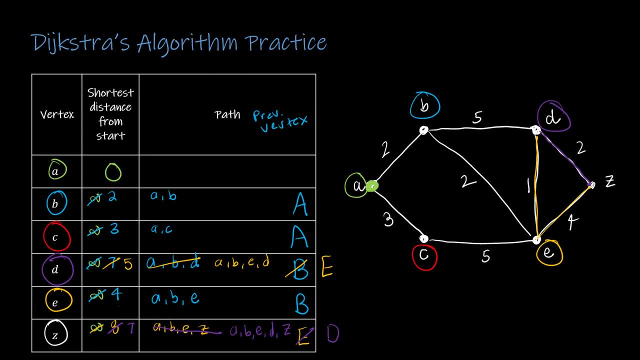 i found the cheapest path to each of these vertices, so so if i needed to get from a to d, the cheapest is five, with a, b, e, d is the path. or again, if you're just looking at the previous vertex- so if you're just showing this, you can find the path to the previous vertex of the previous. 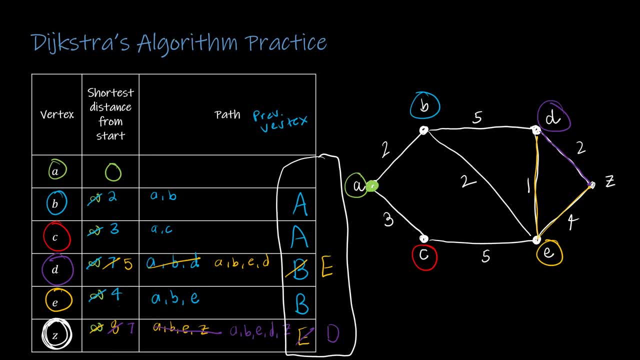 vertex and you would just do this. i'm going to show it to you now so you can see the way it goes. okay, so what we did was we looked at this product and we did a little bit of backtracking and we had to do some backtracking. so let's say i was focused on z. 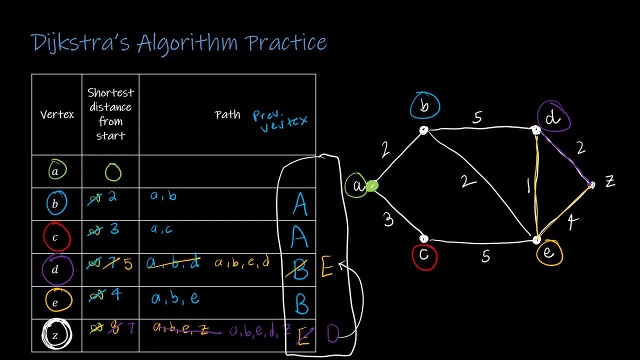 And D said: okay, well, you had to get to E first, And E said you had to get to B first And B said you had to get to A first. So it sort of gives you that path backwards. So up to you if you want to do just the previous vertex or if you want to write out the entire path. 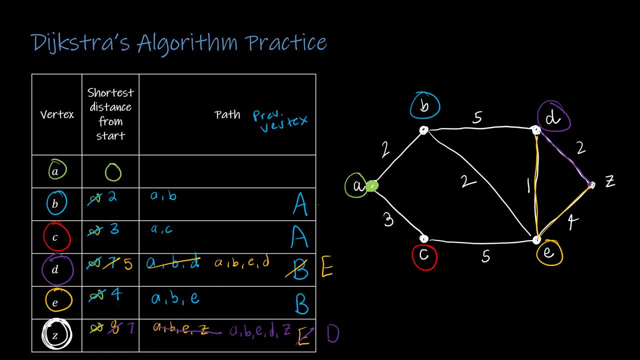 or if you want to show the work on the table or on the graph, You do you, but just make sure that your steps are clear if you are in my class, because I will want to see what steps you followed to find the solution. 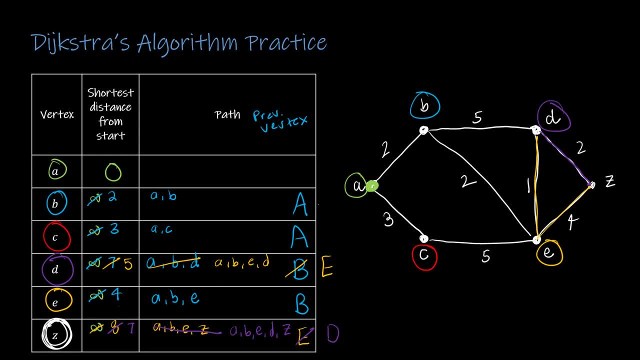 Now, if the question said: just use Dijkstra's algorithm, showing the table would be sufficient, all of the work that I've shown in the table. If it specifically said find the shortest path to Z, then you would say A, B, E, D, Z, and then with a distance of 4.. 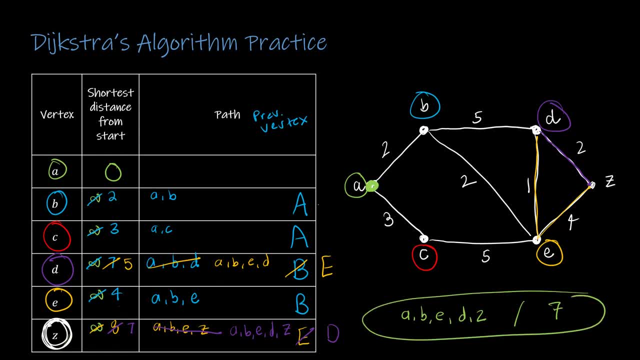 I'm sorry, of 7.. So you You would want to make clear that that was the final solution. Up next, we're going to take a look at graph coloring. 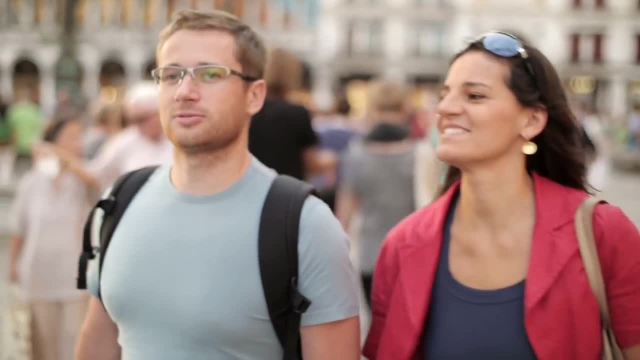 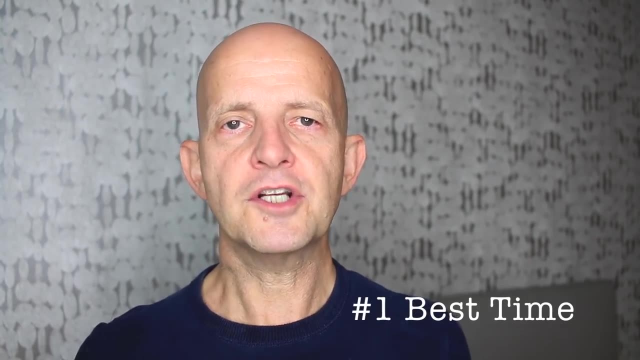 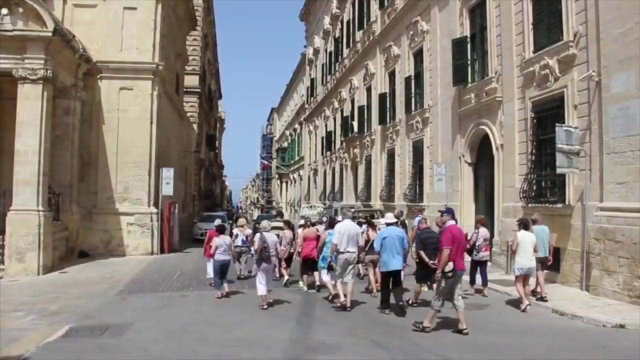 I'm Gary Bembridge of Tips For Travellers. I'm going to give you 11 things that you absolutely need to know to make sure you have an incredible Mediterranean cruise. First of all, when to go Now. the peak season for Mediterranean cruises is from April to October, and, of course, the big big season is July and August. That's when it gets really hot and really expensive. So a really good time, if you can, if you can avoid the school holidays, is to go at the beginning of the season, so May-June time and that sort of September time. That's when you normally have. 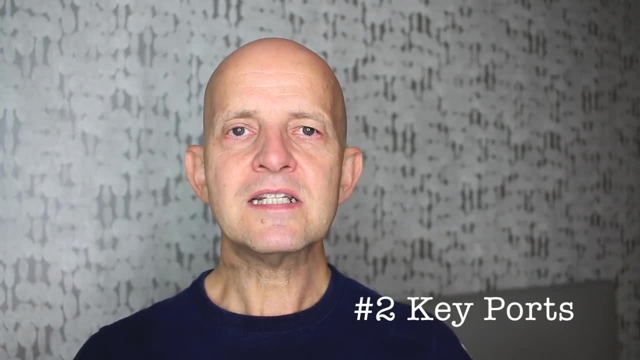 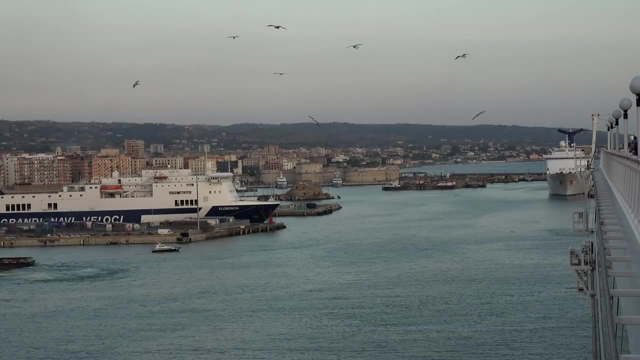 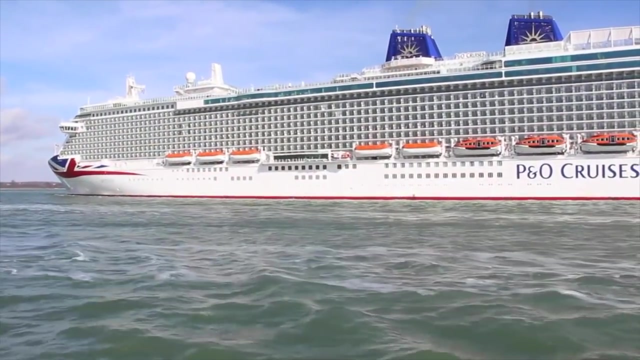 great weather and it's much less crowded. There are six key ports where most Mediterranean cruises depart from: Barcelona, Venice, Genoa, Civitavecchia- which is near Rome- Southampton and Athens. Mostly Mediterranean cruises will leave from those big six embarkation and disembarkation ports. Now one: 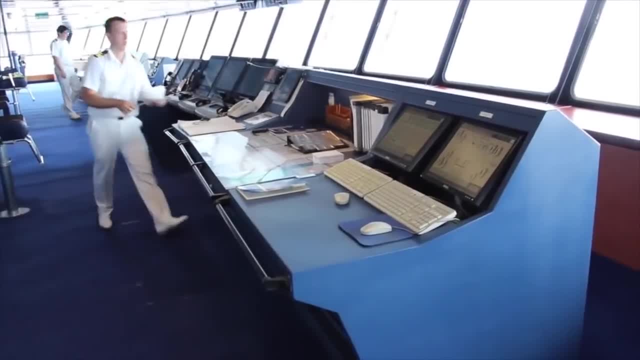 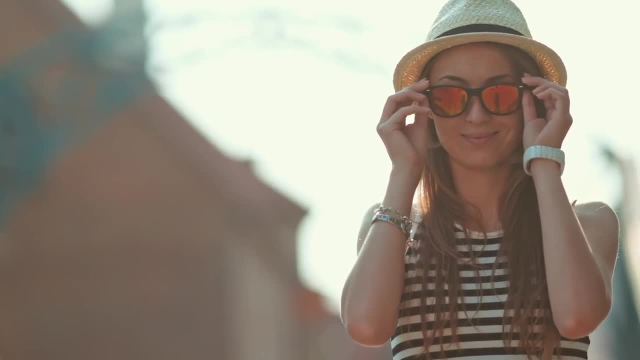 key tip that I have is focus on the ports that actually are within the Mediterranean, because that means that a lot of Mediterranean cruises depart from those big six ports. From the day that you start your cruise, you're in the Mediterranean and there's no transit time.